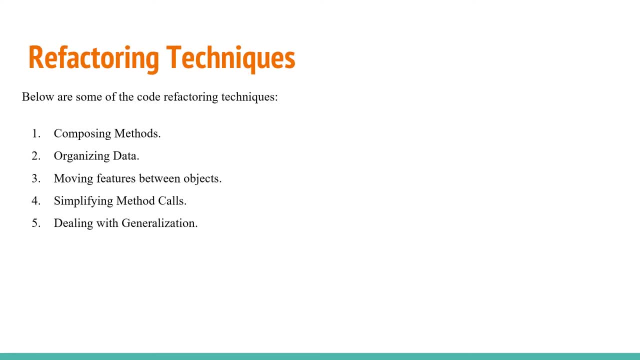 maintainability. Refactoring techniques. Below some of the code refactoring techniques we have composing methods, organizing data, moving features between objects, simplifying method calls and dealing with generalization. In this presentation I'll be focusing on the first two: composing. 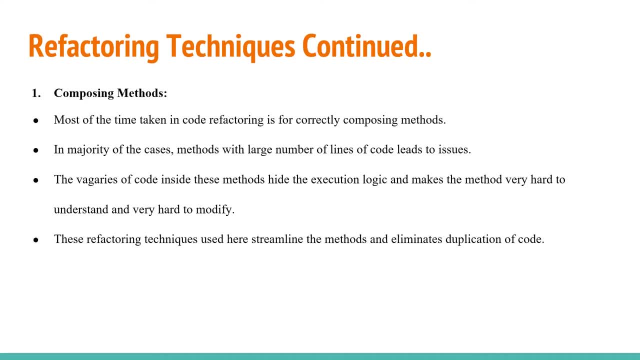 methods and organizing data. Composing methods: Composing methods properly takes most of the time in code. refactoring Methods with large number of lines of code lead to issues. in most of the cases It makes it very hard to go through the code, understand it and to modify it. The refactoring 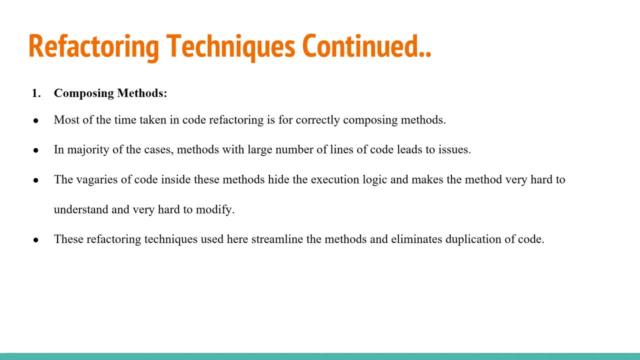 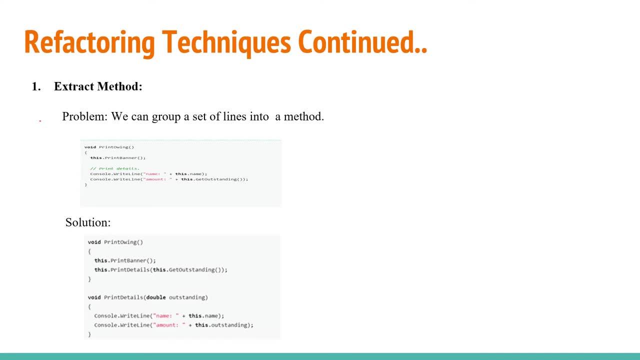 techniques used here streamline the methods and eliminates code duplication. The first one in composing methods is extract method. So this is the code before refactoring and this is the code after refactoring. So what is the problem here? The problem here is we have a set of lines of code. 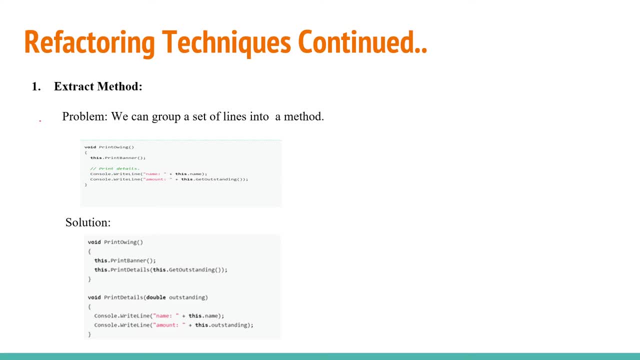 which can be placed inside a method. We have two lines here, but what if we have 10 to 20 lines of code that are repeated at multiple places? Then it is good to place those lines of code in a method and replace the places where we have these lines of code with this method. For example, here, these two: 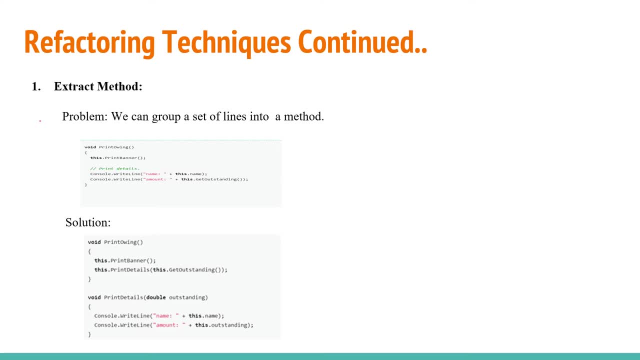 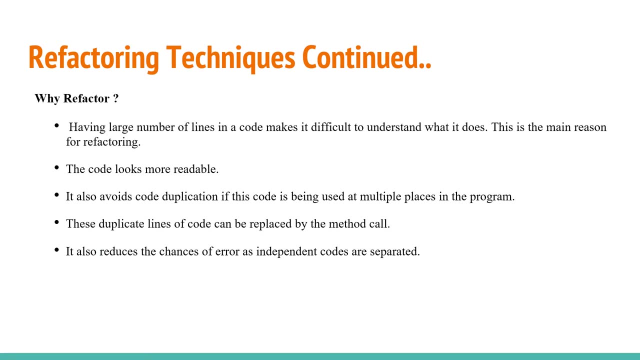 lines of code were placed inside the method and we are calling this method instead of specifying those lines of code inside a method. As a result, this method resource will not be РEFACROMPTED instead of specifying those lines here. so why do we need refactoring? here it is. 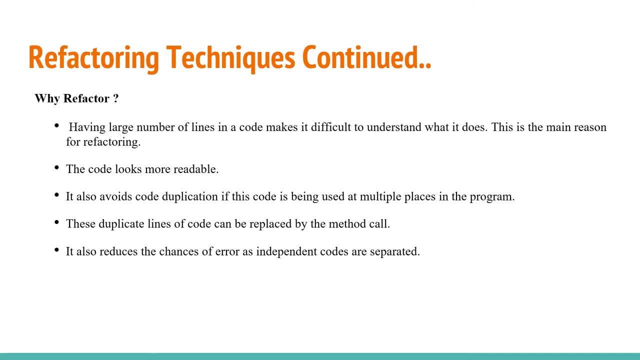 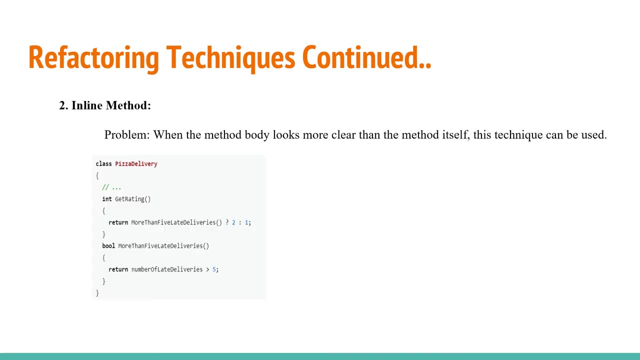 very hard to understand what a code does if there are a large number of lines in code. this is the main reason for refactoring. it makes the code look more readable, it avoids duplication of code and it also reduces the chances of error as independent codes are separated. the second method is inline method, so this: 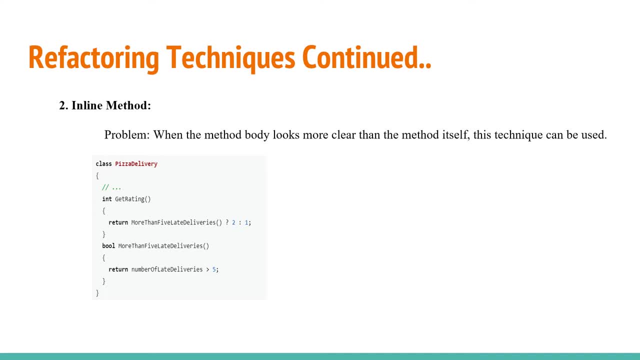 is the code before refactoring. if you see the code, we have a method called get rating and this method is calling another method called more than file deliveries, and this method is returning true or false, based on some condition and based on the result written by this method, it either returns two or one, so 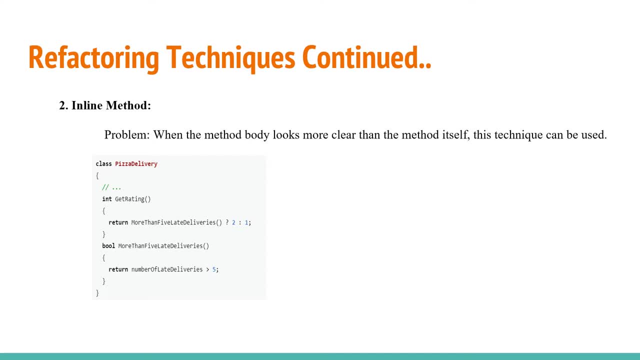 if you observe the method more than file deliveries, the method body looks more obvious than the method. so we need to replace the method call in get rating method with this method body. so this is how it looks after the replacement. so we replaced the code inside the method late deliveries directly with the method body. 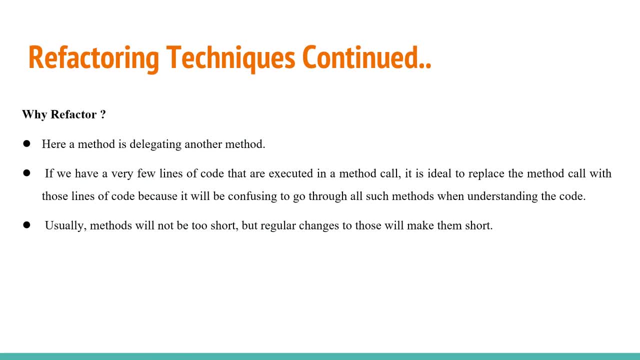 so why do we need refactoring here? so here a method, it's just delegating to another method. so whenever we have a method that has only very few lines of code, like one or two lines of code- and whenever it's returning some value, it is always recommended to replace those method calls with the method body. 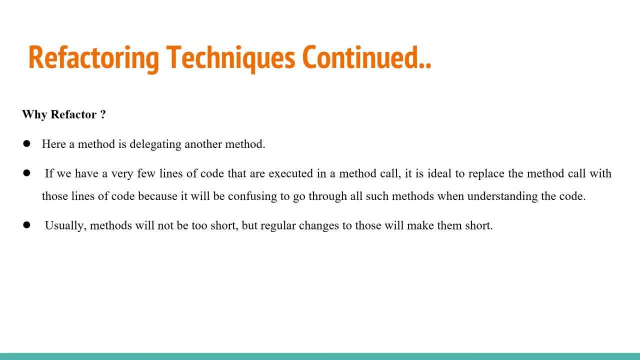 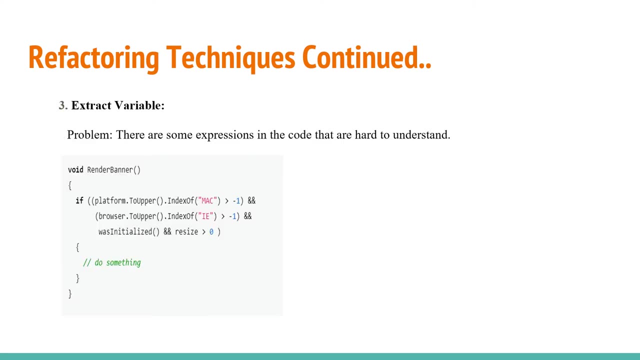 because having a large number of methods like that make its confusing to go through all the code and to understand it. usually methods will be short. sorry, usually methods will not be short, but frequent changes to those methods make them short. the third is extract variable. so the problem is there will be some. 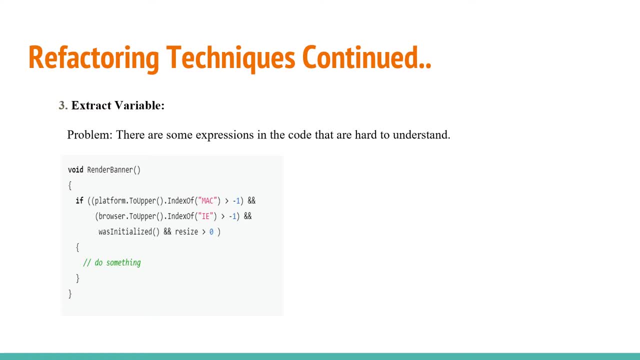 expressions in the code, and soon they're going to change the name of the code. so the problem is that if the numbers are short, it doesn't mean that there are enough solutions, and then the machine will correct itself, probably, and so if there aren't, which are very hard to understand, for example, if you see the code: 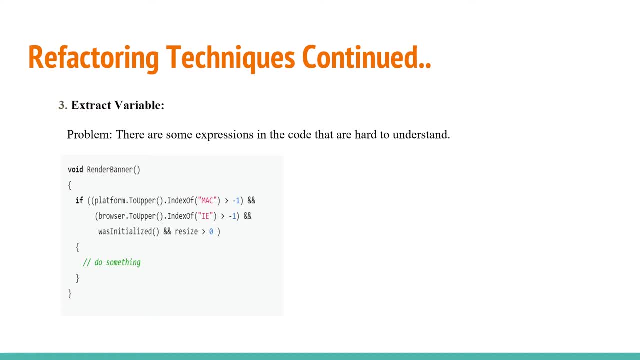 we have like three expressions: platform dot to upper dot, index of mac and two more expressions. so by seeing this we can say that they're quite a bit hard to understand. so the solution is break those expressions, place those results in variables like meaningful variables and use those variables in the if. 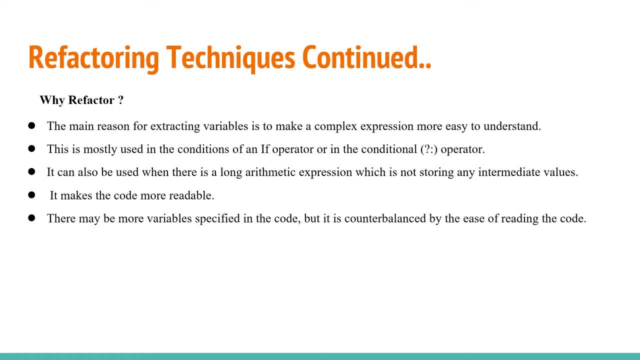 condition. so why do we need refactoring here? the main reason for extracting variables is for making complex expressions easy to understand, so we mostly use this method whenever we have like- if operator or conditional operator and if they're using some conditions in that, we can also use this. 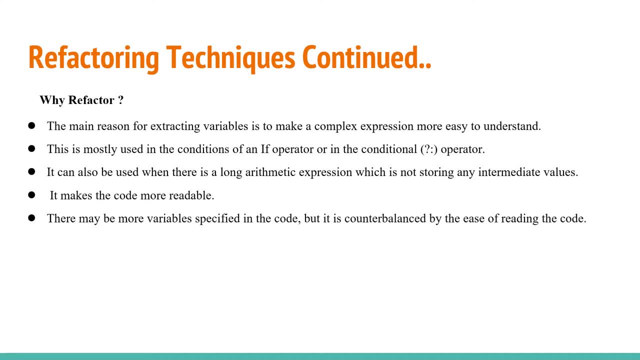 when there are long arithmetic expressions which are not storing any intermediate values. this makes the code more readable. there may be a large number of variables that will be specified in the code if you follow this algorithm approach, but it is counterbalanced by the ease of reading the code. 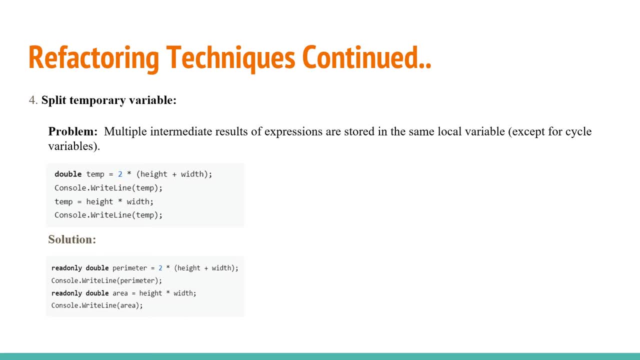 the next method is pre-temporary variable. so this is the method before refactoring. if you see this method, we have a variable called temp and we are using the temp variable to store the value of a result more than once. that is, we are storing the two into height, into width value, into 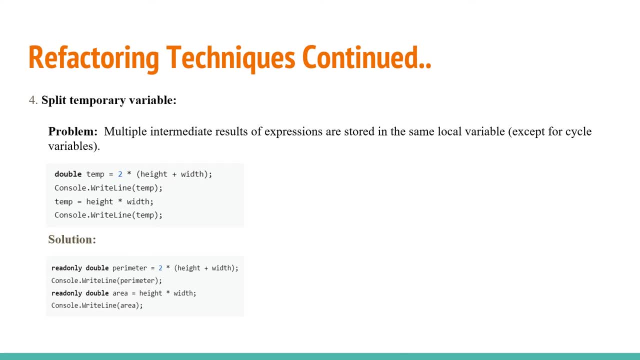 temp. and again we are storing the height into width value into temp. so this is not a good practice. so the good practice is to use these methods for good way, or the solution is to place those results into meaningful variables like 2 into height. height plus width is perimeter. 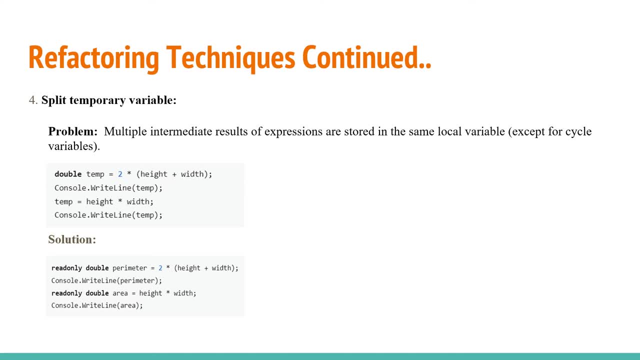 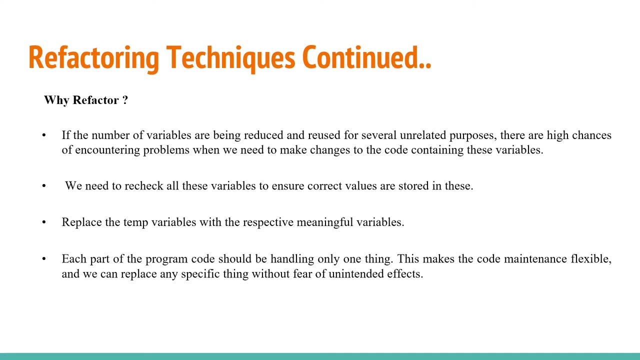 so we are placing in perimeter variable. and height into width is area, so we are placing it into area variable. so why do we need to refactor here? if you are trying to reduce the number of variables for unrelated purposes, then issues may occur if we try to make changes to the code that has these. 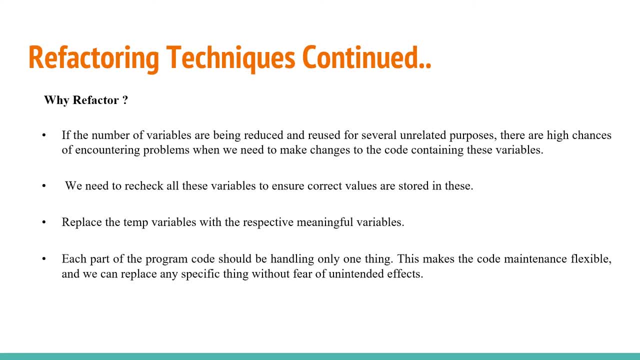 variables. all these variables should be rechecked to make sure they are storing the correct values, and each part of the code should handle only one thing. this makes the code maintenance flexible and we can replace anything without worrying about the unintended unintended effects. the fifth is substitute algorithm, so sometimes 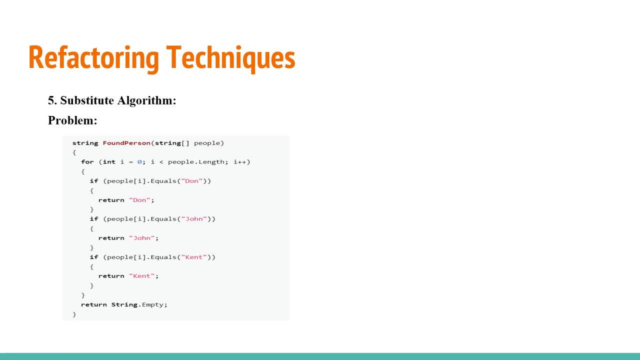 the method is so cluttered with issues such that it is better to replace it with an intended solution rather than a new logic. so if you see this code, it is accepting a stringer as input and it's it is checking for each user whether his name is present in this array or not. 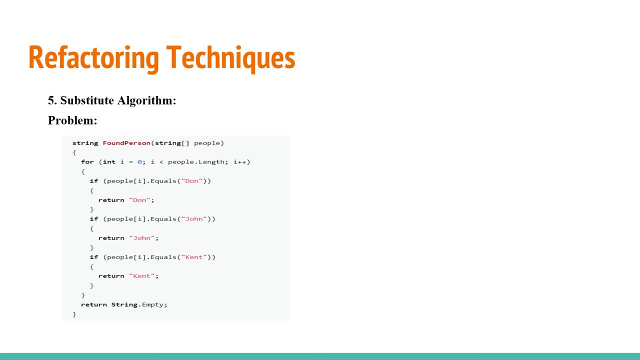 for example, it's checking whether don is in this array list or not, it's checking whether john is in his array list or not, and so on. so this method will become very lengthy if you have a large number of users to check. so it's not a good way of writing the. 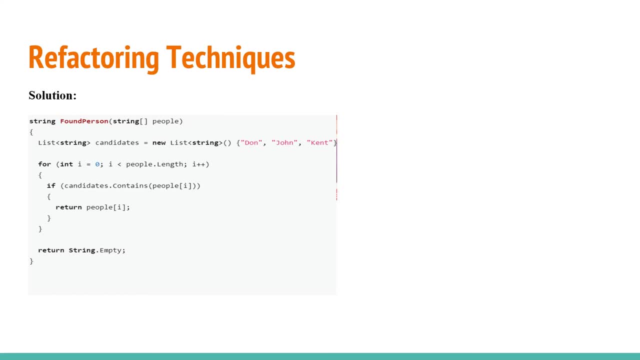 code. the sixth method is to create a list with string type and add all the names that we'll be looking into this array and we can use a c sharp method called contains to check whether these names were in the array or not. so why refactoring? as i said, sometimes the method will be clustered. 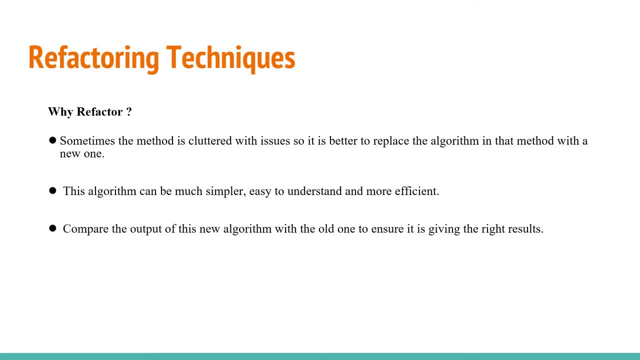 with issues so that it's better to replace that method with a new method. the algorithm will look much simpler, it will be easy to understand and it runs much efficiently. there may not be that significant impact on the performance, but the length of the code will be reduced and we need to compare the output of this new algorithm. 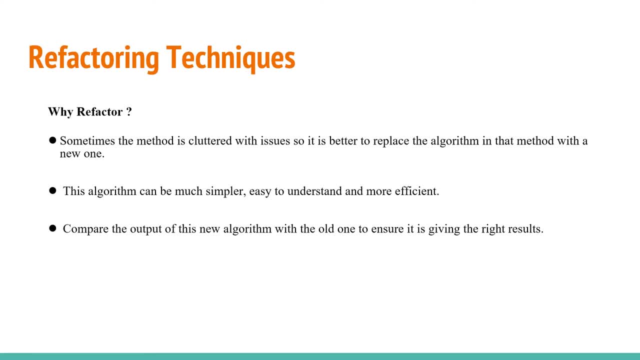 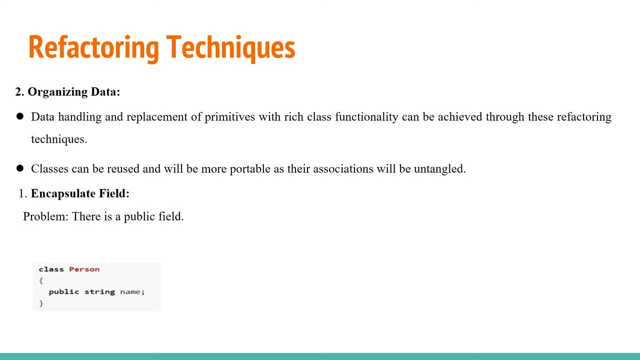 generated with the old one, to make sure the new code is working as expected. the second refactoring technique is organizing data. we can perform good data handling and can use rich class functionality instead of primitive using these refactoring techniques. the first one is encapsulate field. the problem is here. 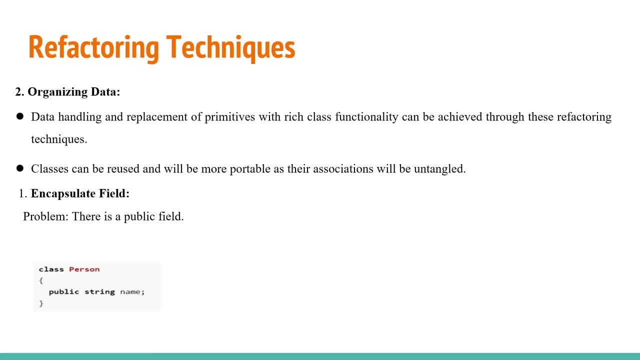 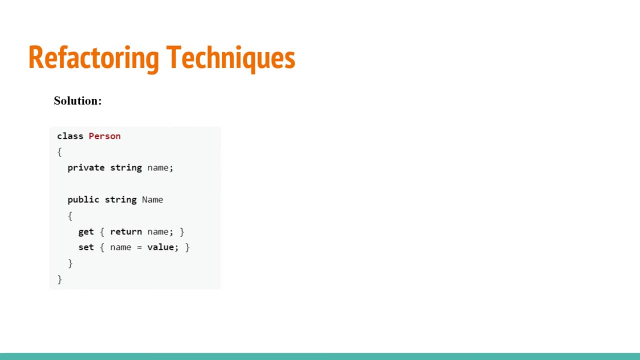 we have a field called name and it is public in this class. so it is not a good way to keep the fields in a class as public. so the solution is we need to create a getter and setter for that variable and we need to make that variable as private. 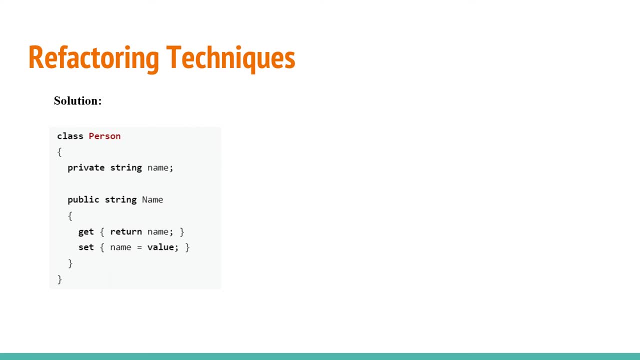 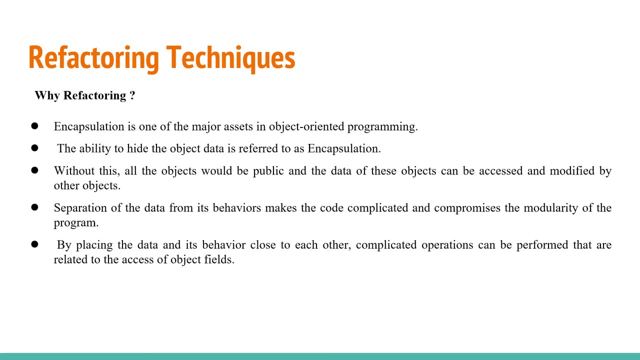 and the variable can be. variable value can be assigned using the setter and the variable value can be retrieved using the getter. so why do we need refactoring here? for object oriented programming, encapsulation is one of its major assets. the ability to hide object data is referred to as encapsulation. without encapsulation, all the objects 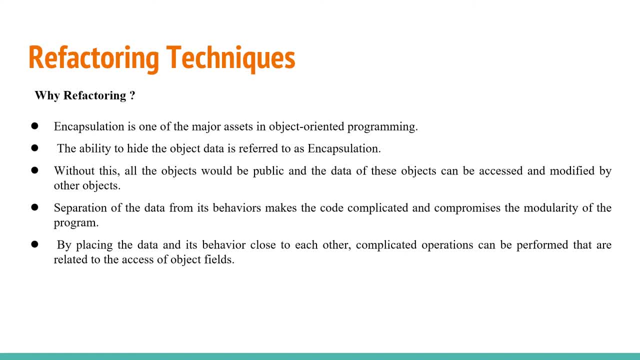 can be accessed and modified by other objects because they will be public. the modularity of the program will also be compromised, as the data will be stored in the getter. the data is separated from its behavior and it also makes the code complicated. so if you place the data and its behavior together, 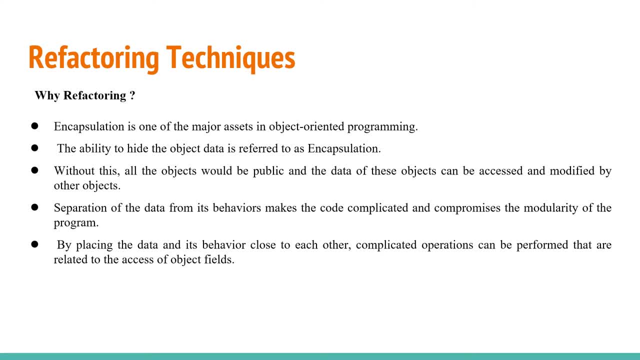 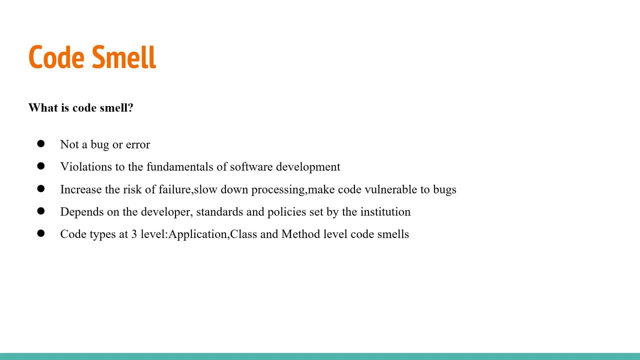 then we can perform better complicated operations that are related to the access of object fields. hello everyone, my name is pushpita and i will give you a walkthrough of what code smell is and types of code smells. a code smell is not an error or a bug, as the code will still do the job. 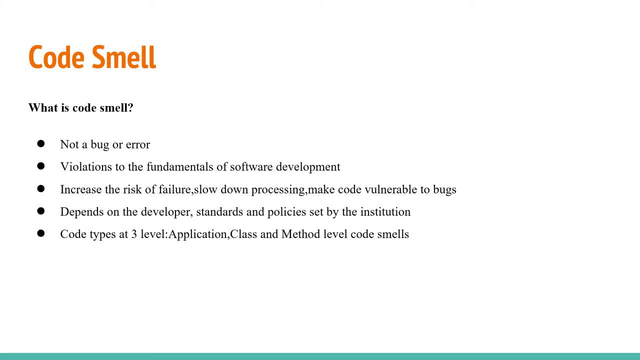 however, the code smell is not an error or a bug, as the code will still do the job. however, they are believed to be absolute violations to the fundamentals of software development that degrade the quality of code. compromising the quality of code might increase the risk of failure, make the code vulnerable to bugs and sometimes, 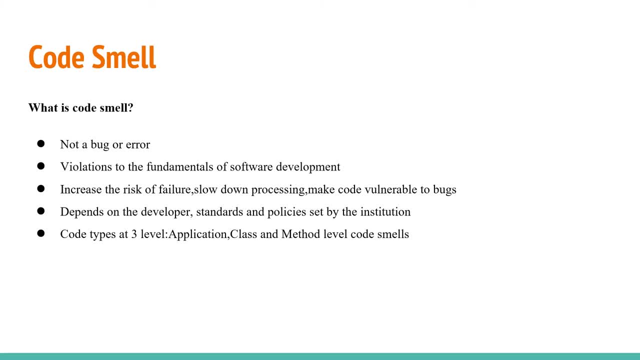 slow down the processing over time. there are different types of code smells. nature of each code smell depends on two factors. first, developer style of programming. second, standards and policies followed by the institution. in the following slides, i will be talking about code smells at application class and method level. 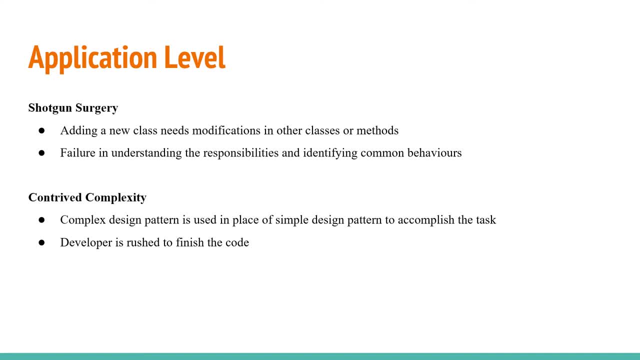 let's look at code smells at application level. at application level, we will be looking at two code smells: shotgun surgery and conserved complexity. shotgun surgery: in this, a developer needs to make modifications in many other classes or methods and or methods upon adding a new class, usually failure in understanding the 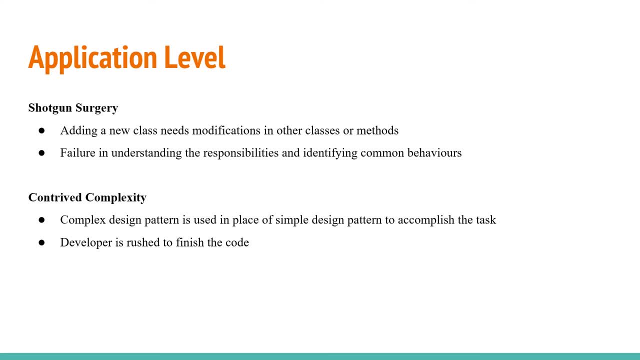 responsibilities in identifying common behaviors lead to shotgun surgery. moving on to conserved complexity, in this, a complex design pattern is used in place of a simple and basic design pattern. the main cause of the situation is where developers are forced to complete code quickly in order to meet deadlines. 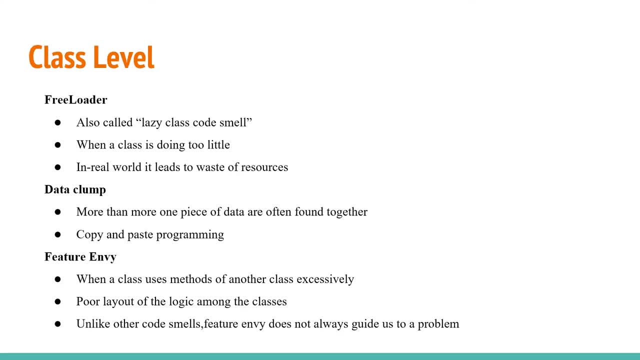 developers are forced to complete code quickly in order to meet deadlines. developers are forced to complete code quickly in order to meet deadlines. moving on to code smells at class level free loader, this code smell is also called as lazy class. this exists when a class is doing too little. 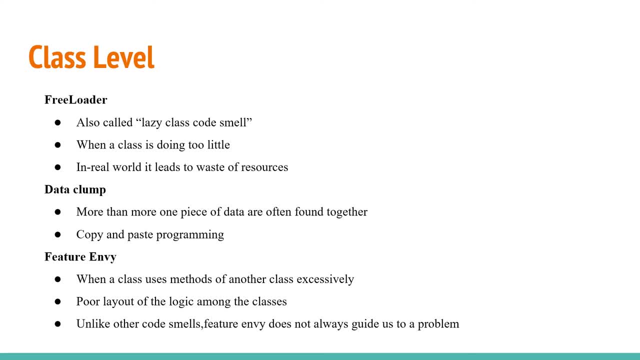 why is this an issue? because in real world, every line of code consumes money and having a class with limited capability only leads to waste of resources. data clump- this code smell speaks for itself. this code smell means more than one piece of data are often found together. for example, if your application maintains employee. 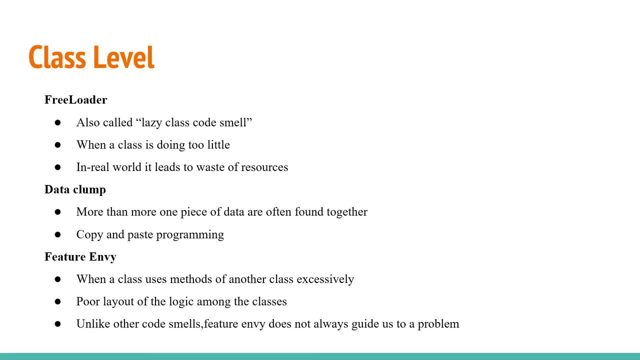 information data like start date of employment and end date of employment would be found multiple times together at different places in the application. this often is the result of following poor programming structure or copy and paste programming feature envy. this code smell exists when a class is using methods of another class excessively. 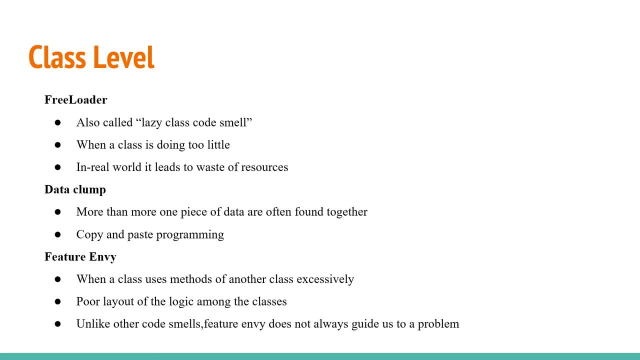 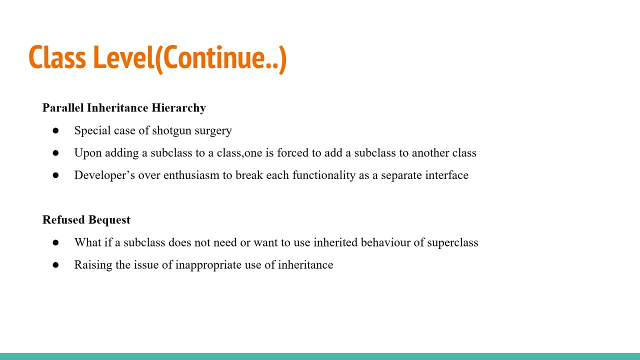 this, again, is a result of poor layout of the logic among classes. unlike other code, smells feature envy does not always guide us to a problem. moving on to parallel inheritance hierarchy, it is a special case of shotgun searching, in this case, whenever a new subclass is added to a class. 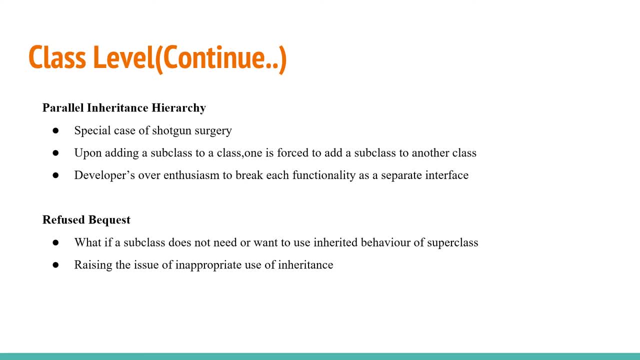 developer is forced to complete a new class. developer is forced to add a new subclass to another classes as well. the trick used here to find this code smell is to look at the prefixes of class names in one hierarchy and comparing it to the prefixes of another hierarchy. 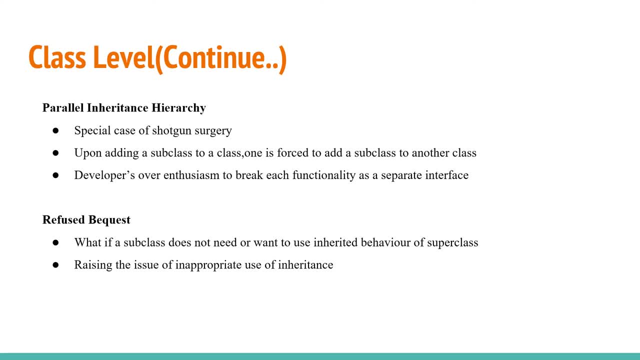 refuse bequest. a subclass has the privilege to use the methods and data of its parents class, but what if the subclass does not need or want to use the inherited behavior? this code smell raises the issue of inappropriate use of inheritance. now let's look at code smells. 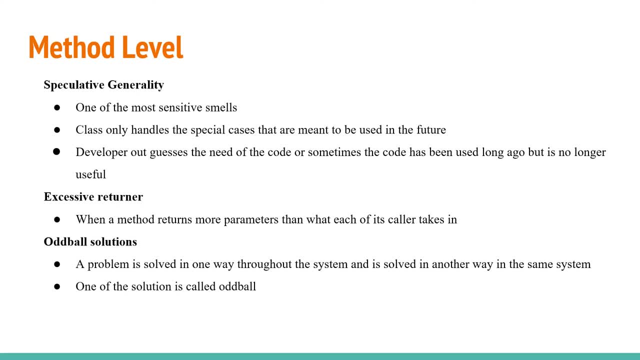 at method level: speculative generality. this smell is believed to be one of the most sensitive smells. this code smell is found when a developer uses a class only to handle the special cases that are meant to be used in the future but might not be useful in at that stage of an application development. 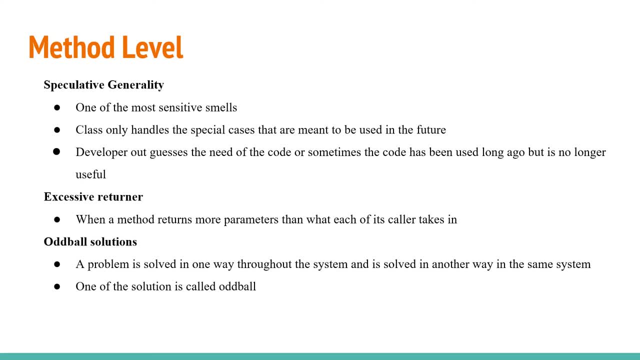 a developer ends up having this code smell in his code when he outgases the need of the code. or sometimes the code has been used long time ago but is no longer useful because of the new ways of doing things. excessive returner refers to a method. 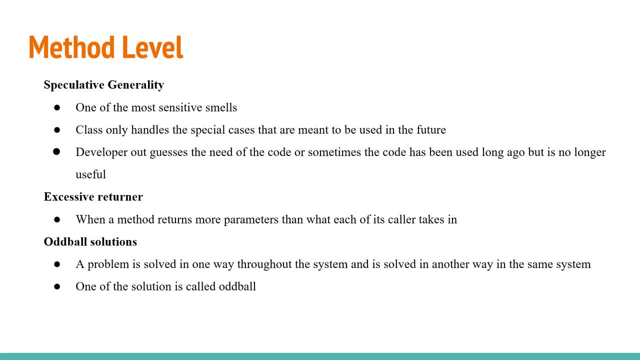 that returns more number of parameters than what each of its caller takes in oddball solution. this smell indicates that a problem is solved one way throughout the system and is solved in another way in the very same system. one of the solutions is called the oddball. in the next slides i will introduce you to the code smells.